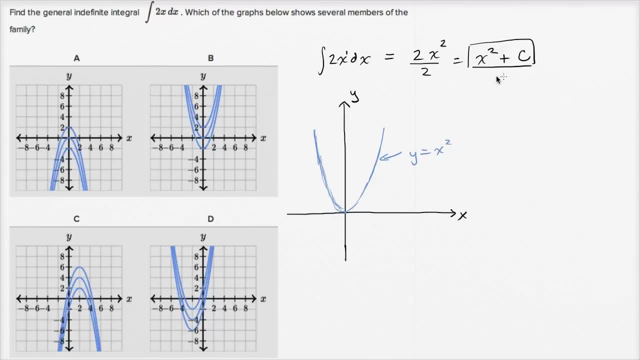 This right over here is: y is equal to x squared. But remember, and I guess you could say that in this case our c is zero. But what if our c was some positive value? So let's say it is: y is equal to x squared. 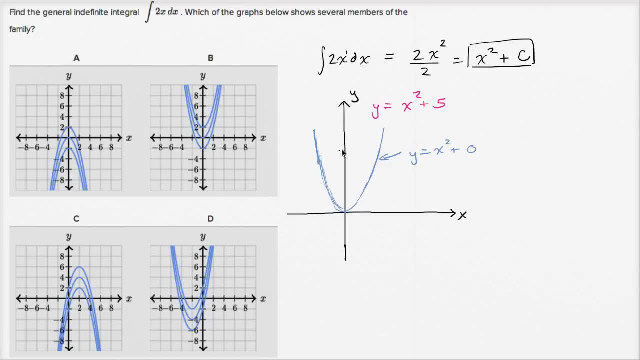 plus I don't know. y is equal to x squared plus five. Well then, we're going to have a y intercept here at five. so essentially, we're just gonna shift up the graph by our constant right over here, which is positive five. 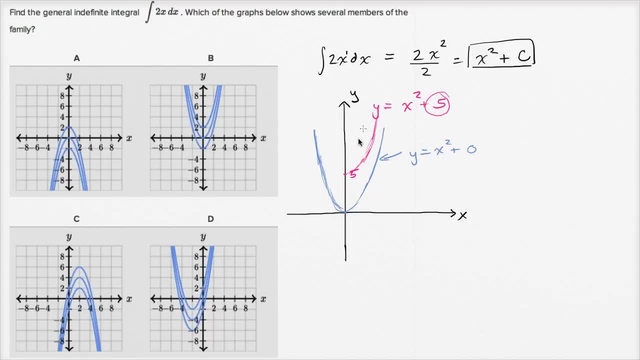 so we shift up by positive five and we will get something that looks like this: We just shifted it up. Now you might be saying, okay, well, that kind of looks like this choice right over here. but this choice also also has some choices that start down here. 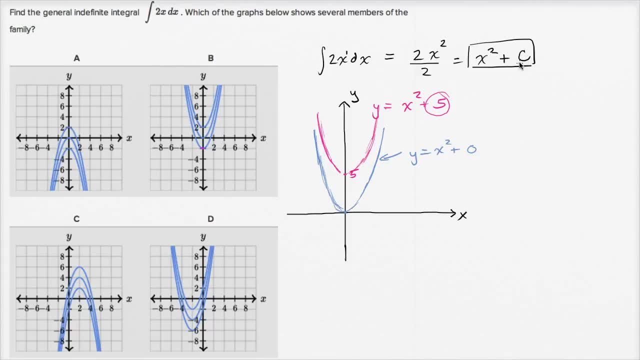 I thought we're adding a constant, but you remember, this constant can be any constant. It could be a negative value. So in this case c is five, in this case c is zero, but c could also be negative five. 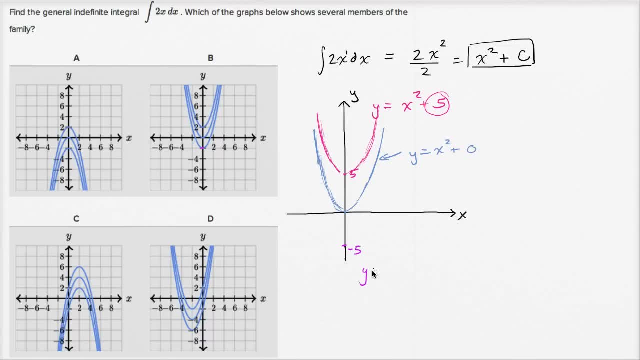 So c could also be negative five. So if we wanted to do: y is equal to x squared plus negative five, which is really x squared minus five, then the graph would look like this: It would shift x squared down down by five. 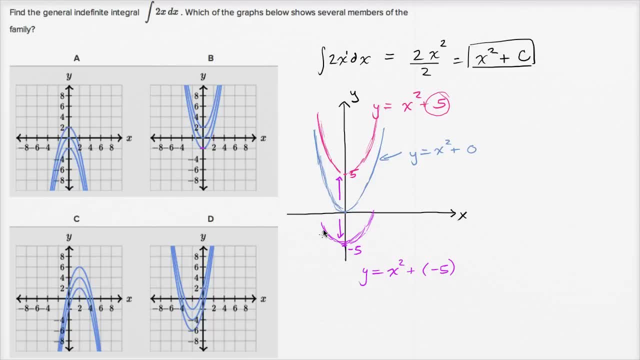 So this one is shifted up by five, this one is shifted down by five. So you would shift by the constant. If it's a positive constant, you're going up, If it's a negative constant, you are going down. So b is definitely the class of solutions. 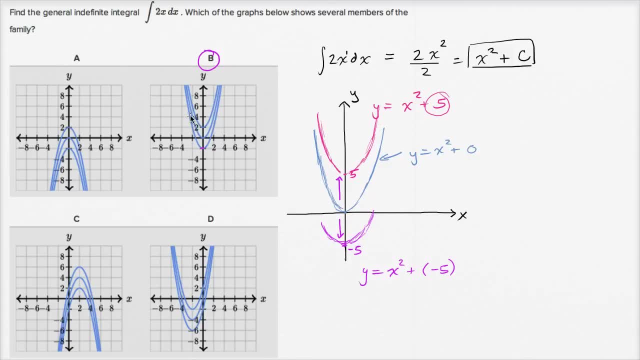 to this indefinite integral. You take any of the functions that are represented by these graphs, you take their derivative. you're going to get two x- Or another way to think about it- the antiderivative of this, or the integral, the indefinite integral of two x- dx. 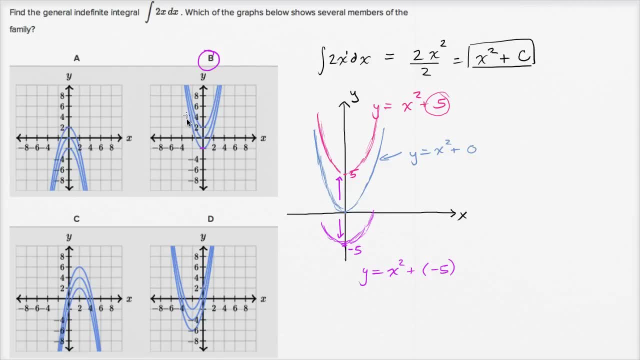 is gonna be x squared plus c, which would be represented by things that look like. so, essentially, y equals x squared shifted up or down. So I could keep drawing over and over again.